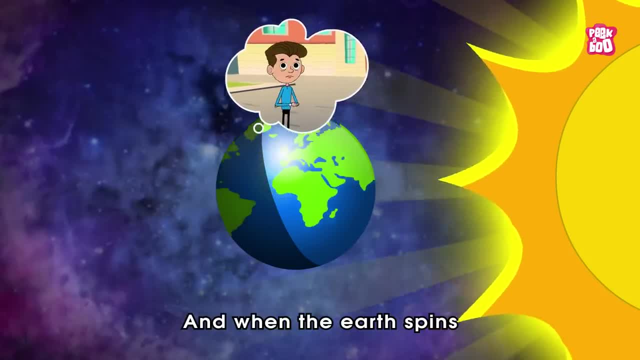 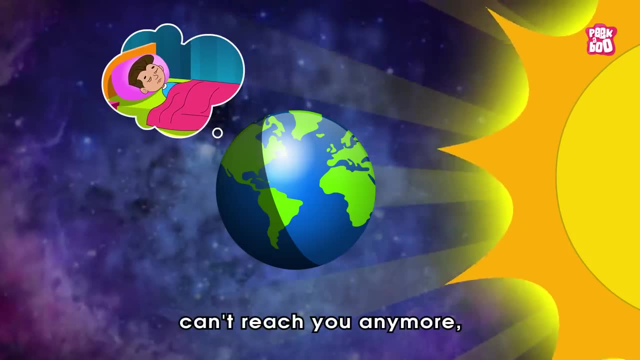 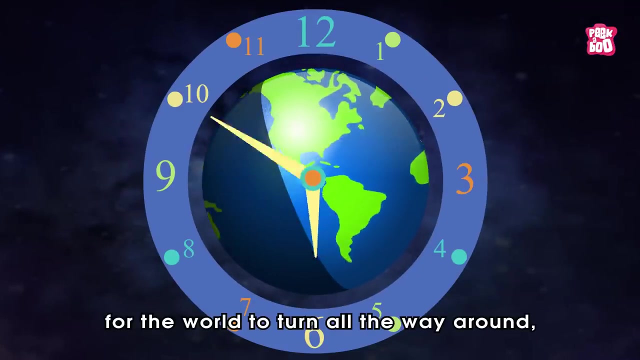 it's daytime And when the Earth spins to take you away from the sight of the sun, where its light and heat can't reach you anymore. it's nighttime And it takes 24 hours for the Earth to turn all the way round to make a single day. 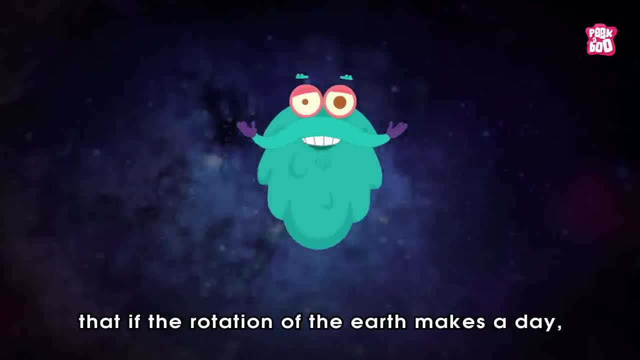 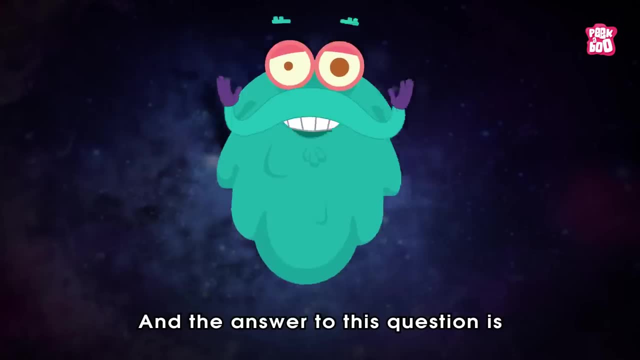 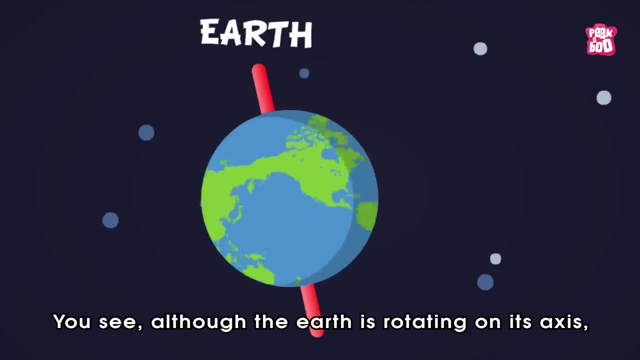 I know you guys must be thinking that if the rotation of the Earth makes a day, then what makes a year? And the answer to this question is the revolution. Let me explain. You see, although the Earth is rotating on its axis, 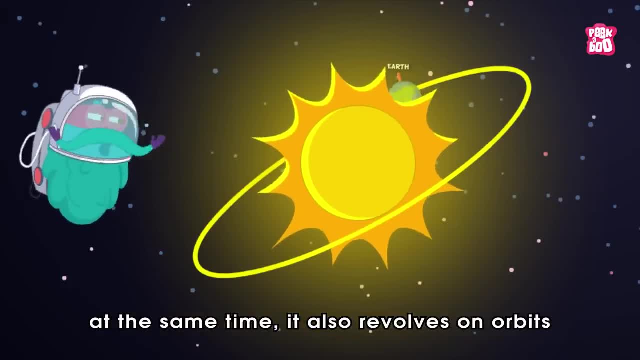 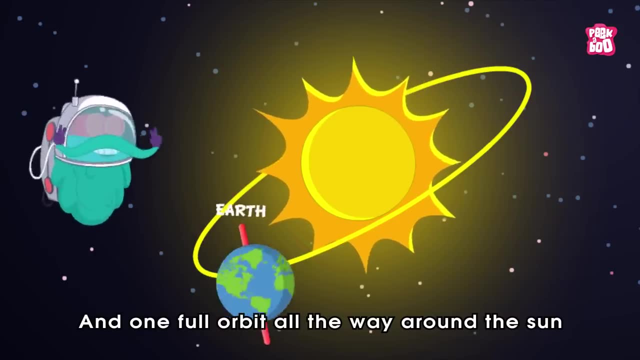 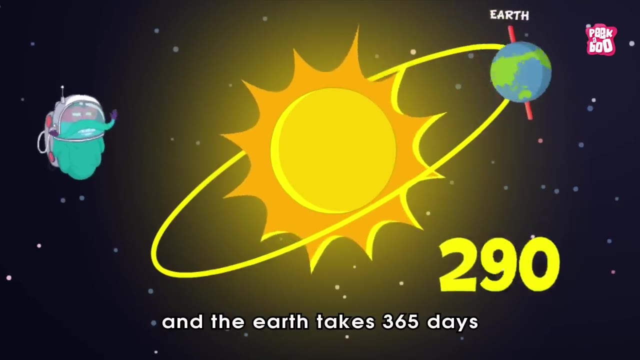 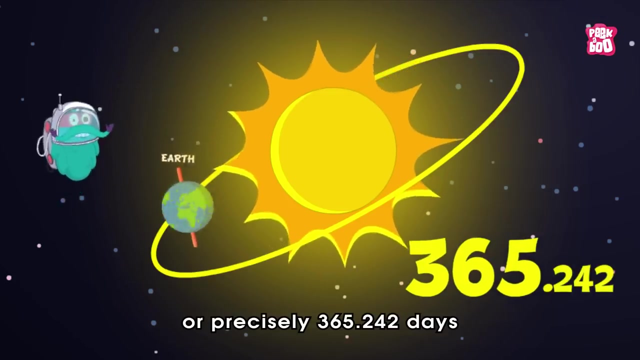 at the same time, it also revolves on orbits around the sun, which is called revolution, And one full orbit all the way around the sun is one revolution, And the Earth takes 365 days, or precisely 365.242 days, to complete a revolution that makes up a whole year. 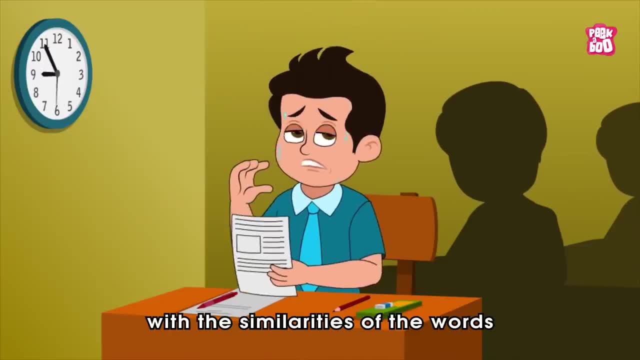 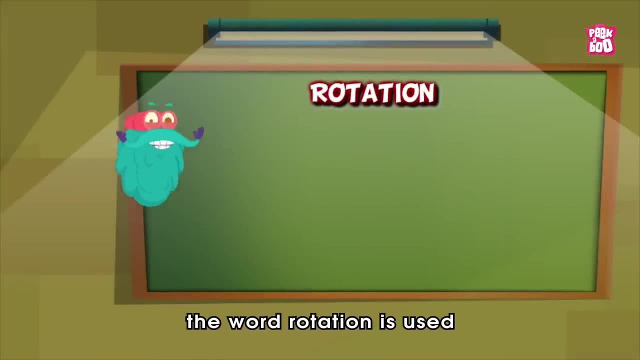 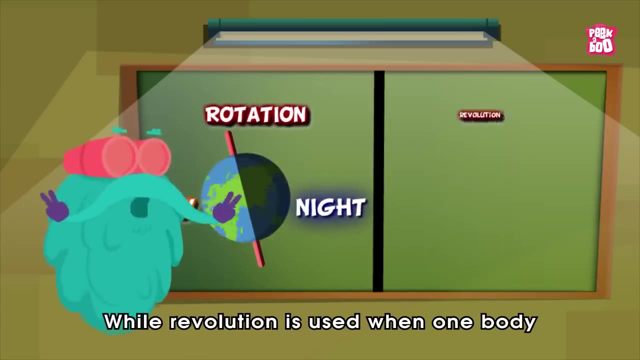 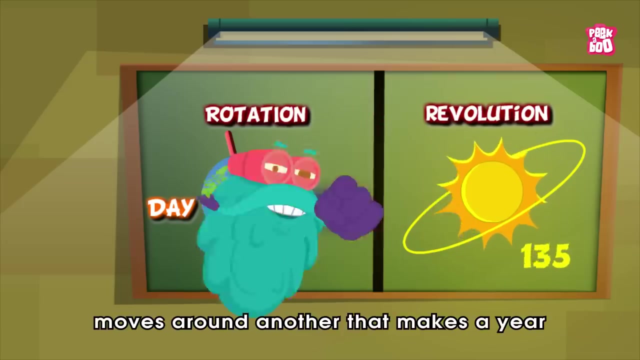 But don't get confused with the similarities of the words rotation and revolution, my dear friends. In astronomy, the word rotation is used to mean the movement around the axis, which creates the day and night on Earth, While revolution is used when one body moves around another. that makes a year. 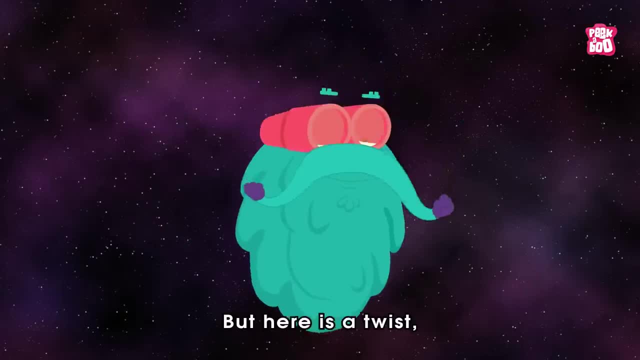 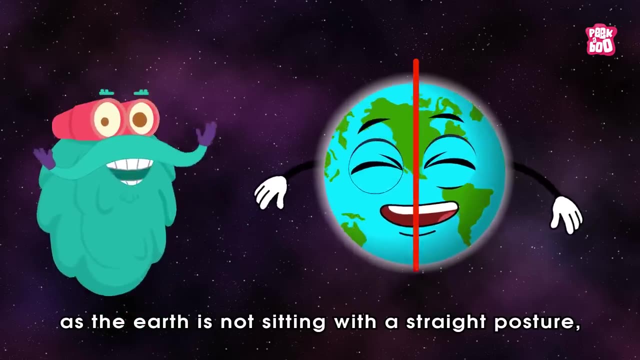 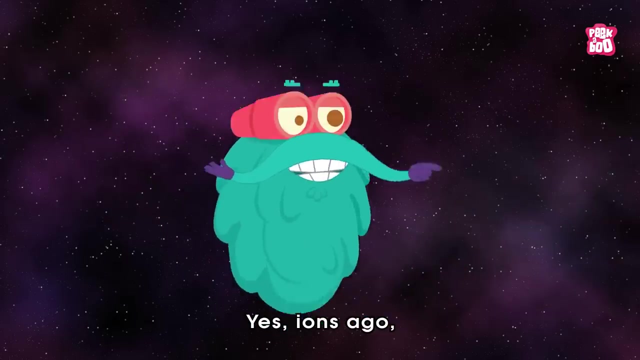 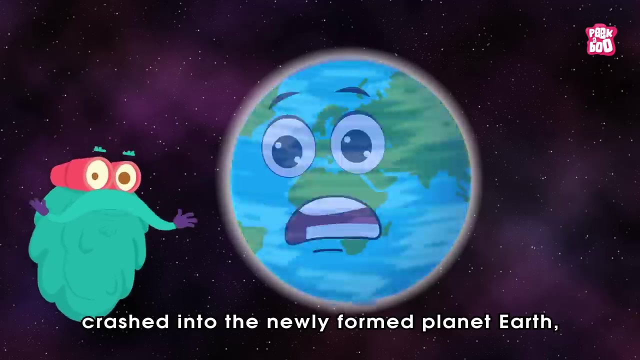 in the case of our planet Earth. But here is a twist, and that twist is in the axis, as the Earth is not sitting with a straight posture, but its axis is actually a little tilted. Yes, ions ago, when an object the size of Mars crashed into the newly formed planet Earth, 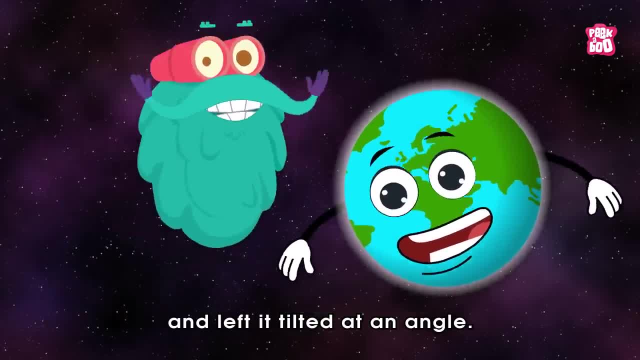 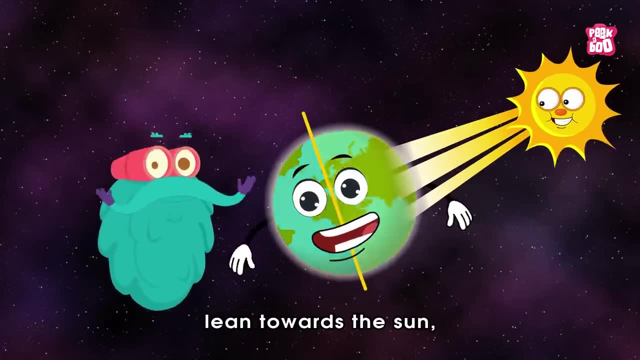 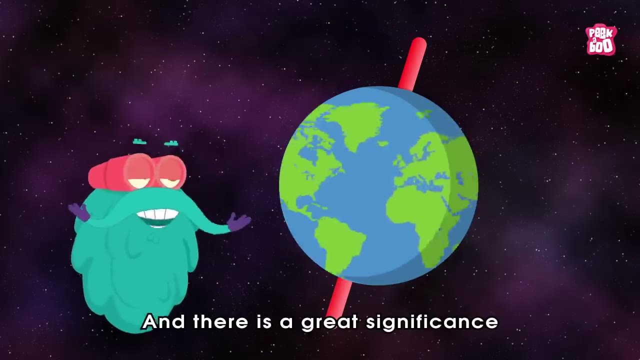 it knocked our planet over and left it tilted at an angle, And this slight tilt made one part of the Earth lean towards the sun, while the other part of it is leaning away. And there is a great significance to this tilt, my dear friends. 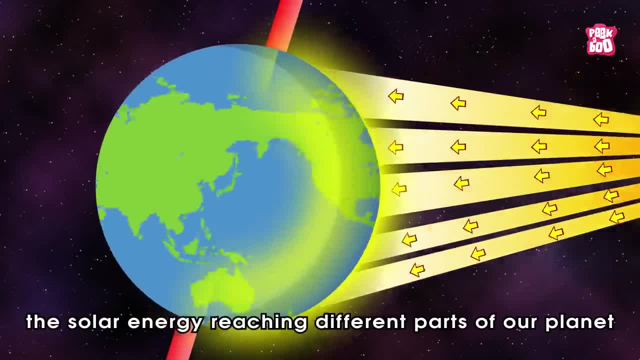 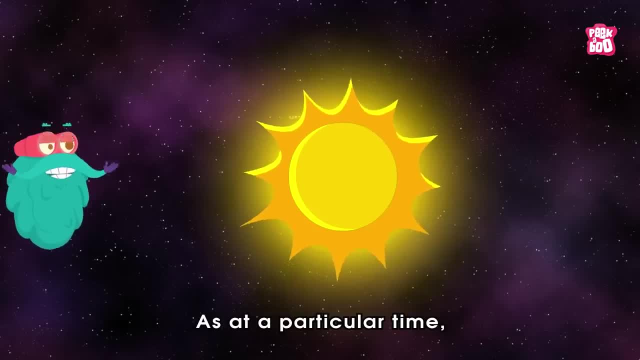 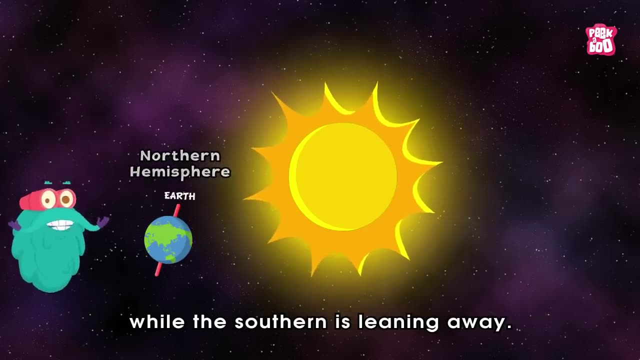 Yes, due to this angle, the solar energy reaching different parts of our planet is not constant, but varies during the year, As at a particular time, the northern hemisphere is leaning towards the sun, while the southern is leaning away, And at other times 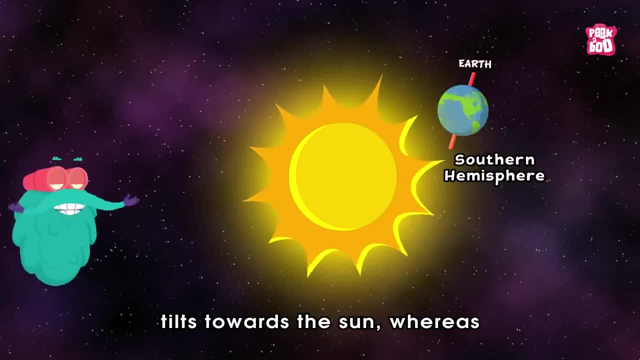 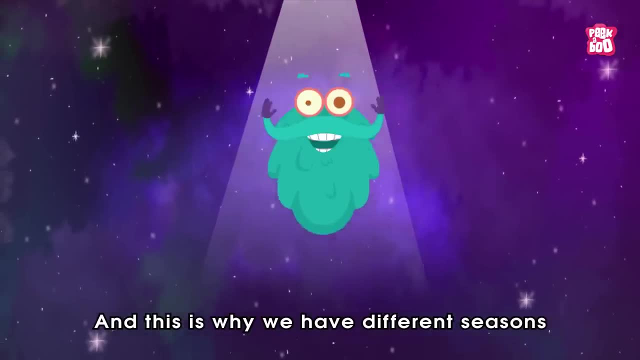 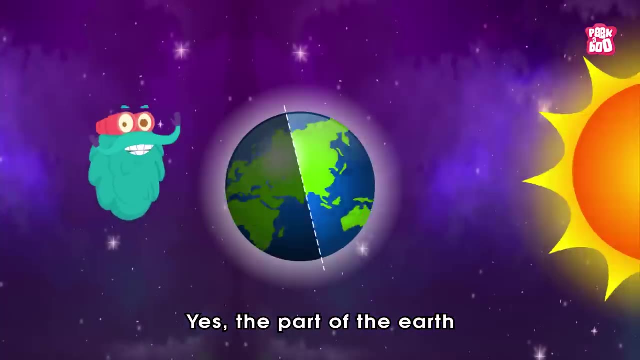 the southern hemisphere tilts towards the sun, whereas the northern hemisphere leans away, And this is why we have different seasons and why the seasons are opposite in the northern and southern hemispheres. Yes, the part of the Earth leaning towards the sun. 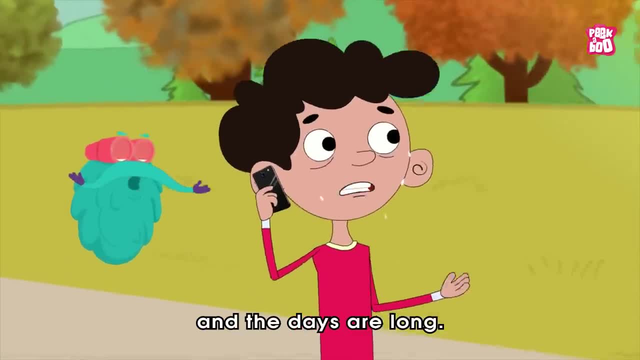 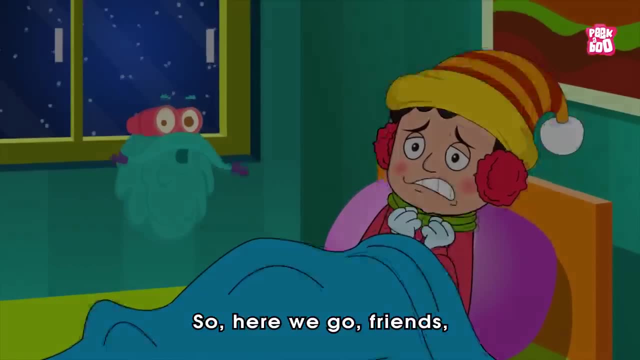 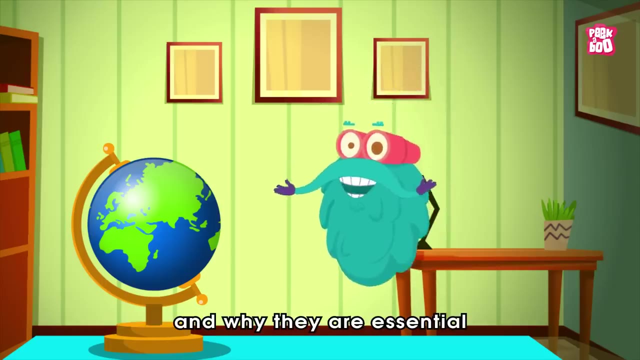 causes summer in that region and the days are long, while the part leaning away experiences cold climate with shorter days. So here we go, friends. Now you know the difference between Earth's rotation and revolution and why they are essential to make your world go round and round. 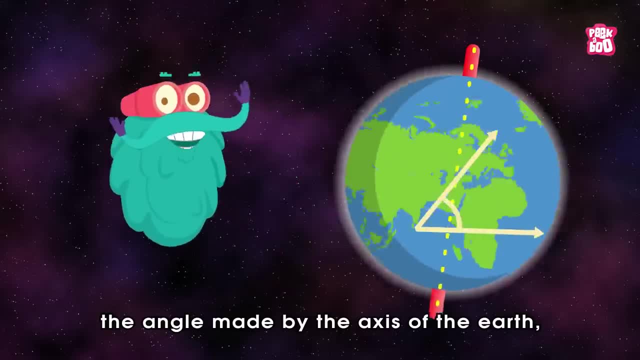 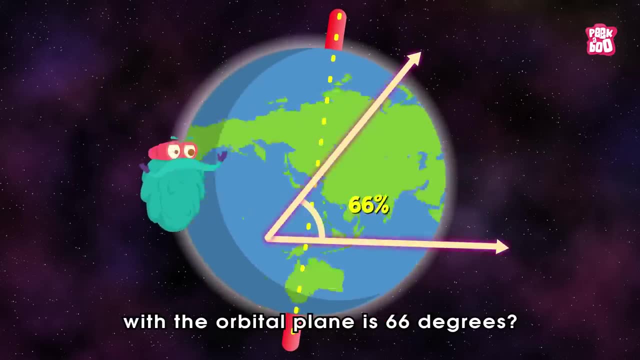 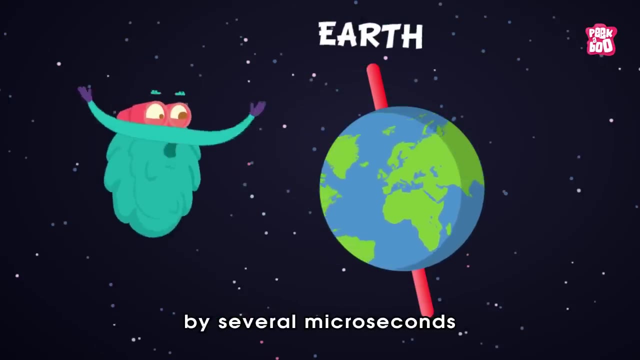 Trivia time. Did you know the angle made by the axis of the Earth, which is an imaginary line with the orbital plane, is 66 degrees. Also, it is said that humans have made a moderate change in the Earth's rotation period by several microseconds. 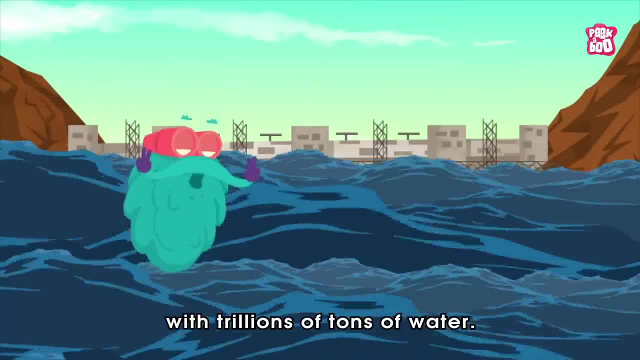 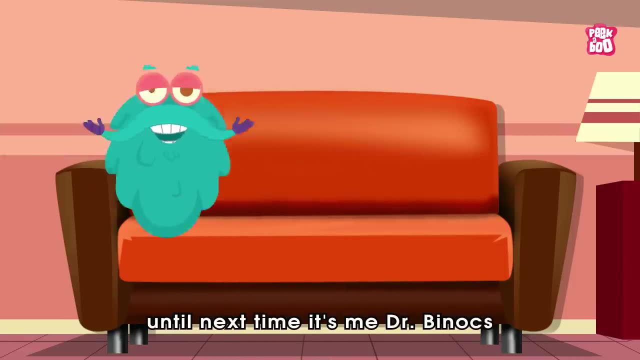 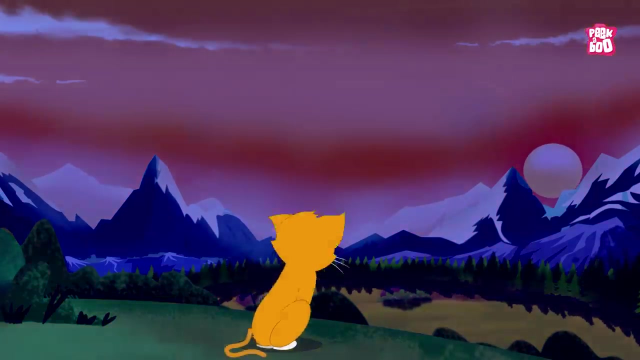 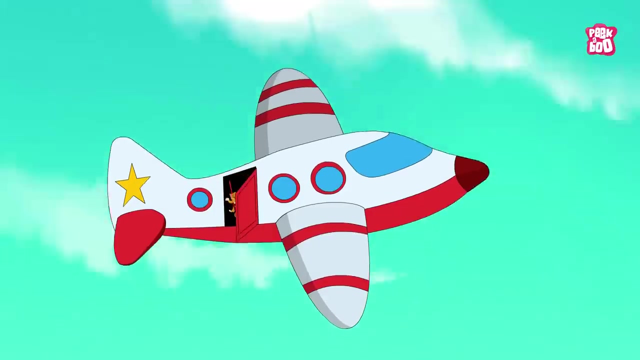 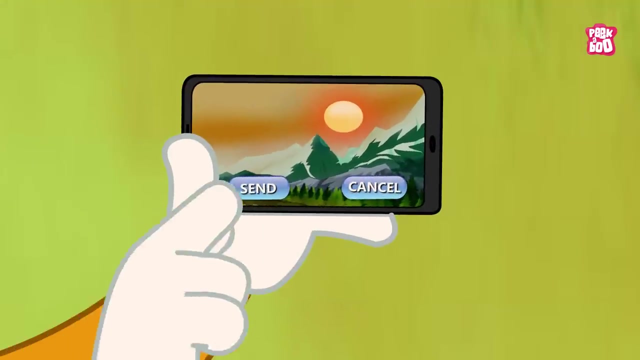 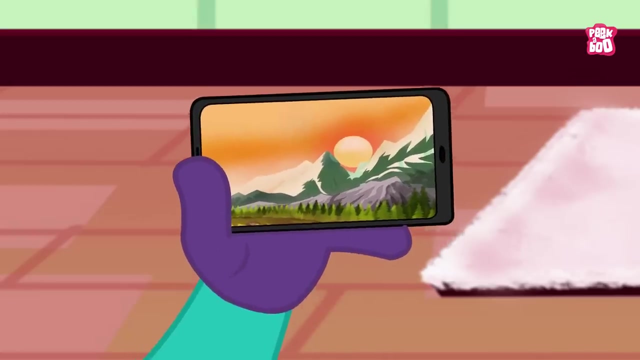 by accumulating vast reservoirs with trillions of tons of water. Hope you learned something new in today's episode. Until next time it's me Dr Binox Zooming Out. Oh, never mind.